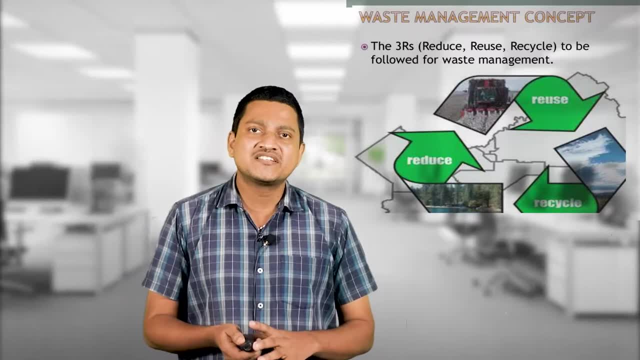 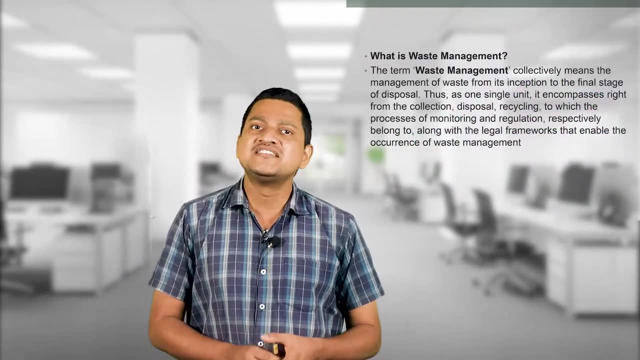 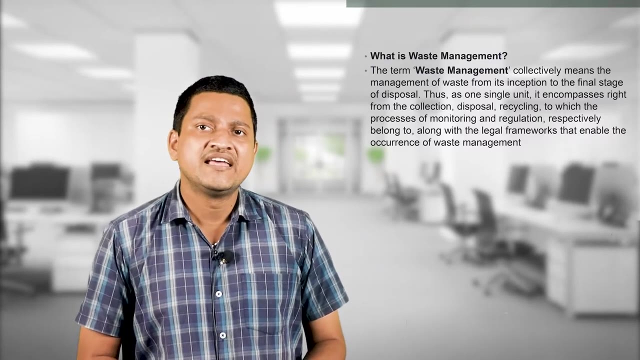 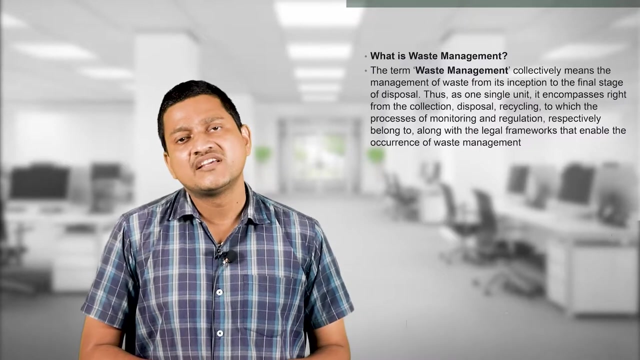 recycle. In this class we mainly focus on these three type of waste management strategy, that is, three R's Waste management is defined. The term waste management collectively means the management of waste from its inception to the final stage of disposal. Thus, as one single unit, it encompass 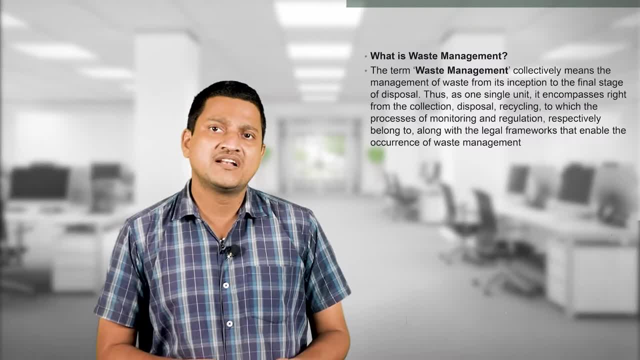 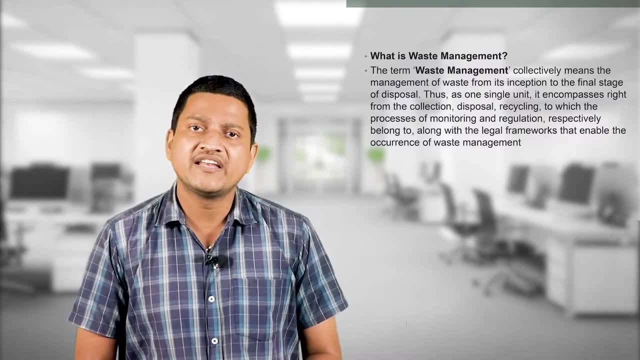 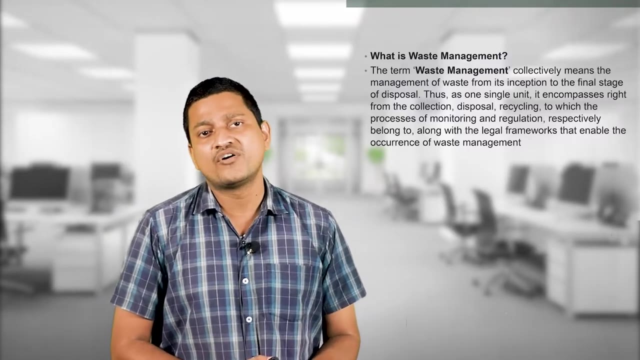 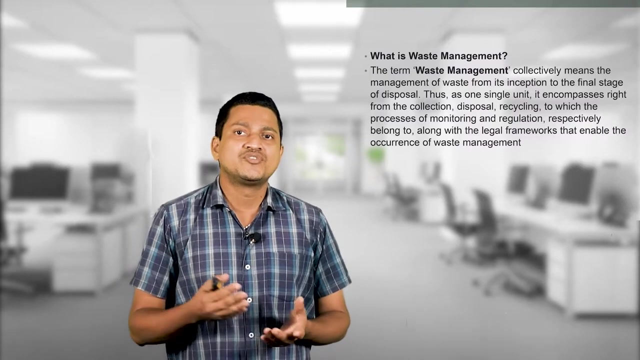 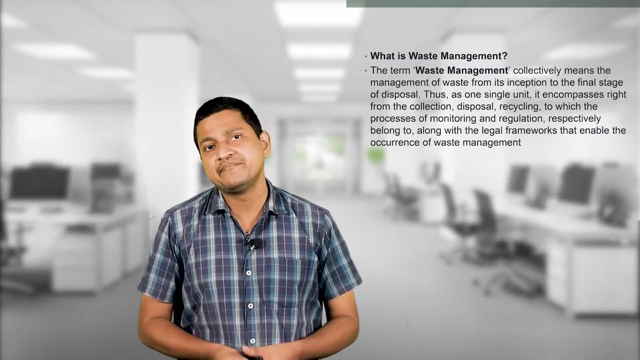 right from the collection, disposal, recycling, to which the process of monitoring and regulation respectively belong to, along with the legal framework that enable the occurrence of waste management, The entire system that, starting from waste generation to disposal, is discussed as waste management. Waste management collectively means the management of waste from its inception to the final stage of. 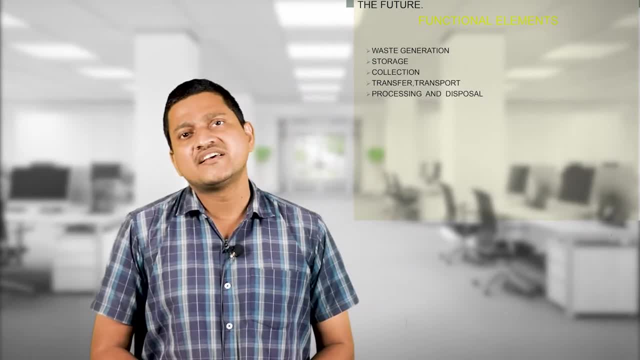 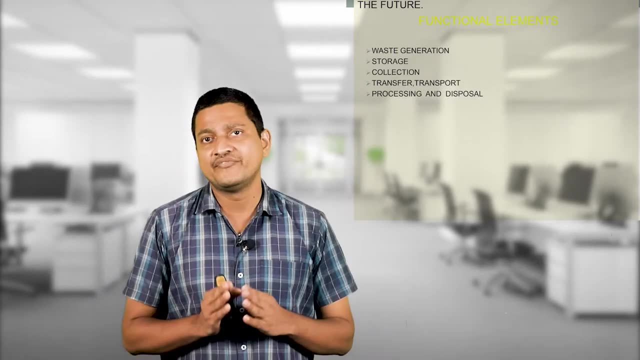 disposal. Next, the solid waste management. short form is SWM, that is, solid waste management. The objective of solid waste management is to manage waste from its inception to the final stage of disposal. In addition to the solid waste management, the fifth objective of solid waste management is to minimize the 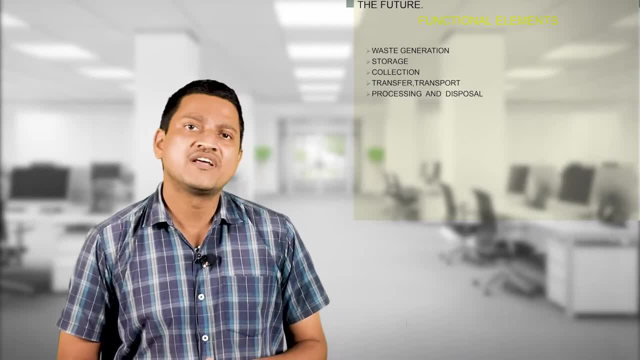 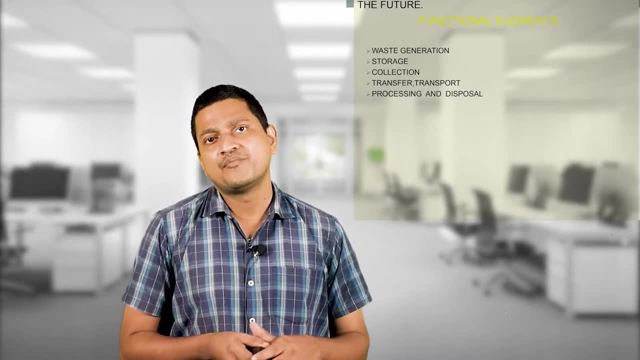 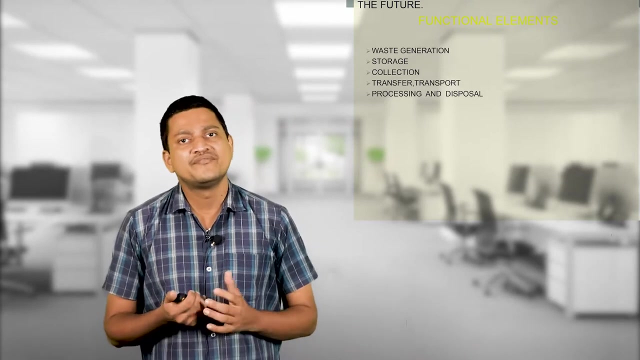 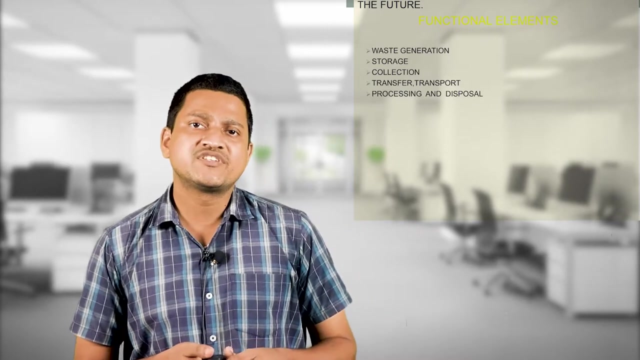 adverse environmental effects before it become too difficult to rectify in the future. That is the main objective of solid waste management. the functional elements of solid waste management, including waste generation, storage, collection, transfer and transport, processing and disposal- These are the main objectives of the taskiminim pictureon. 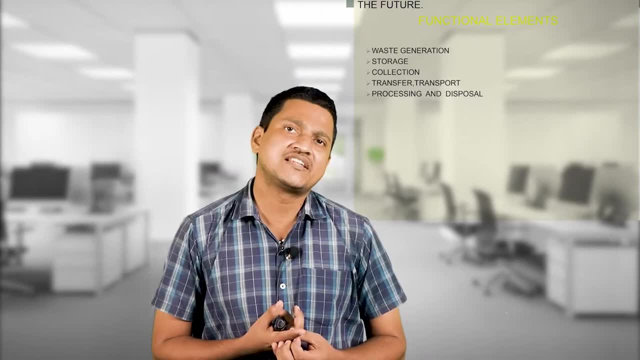 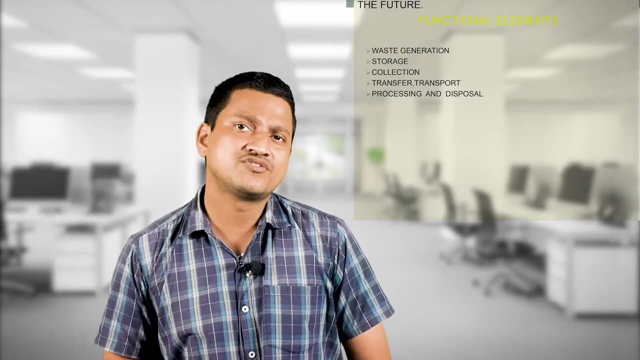 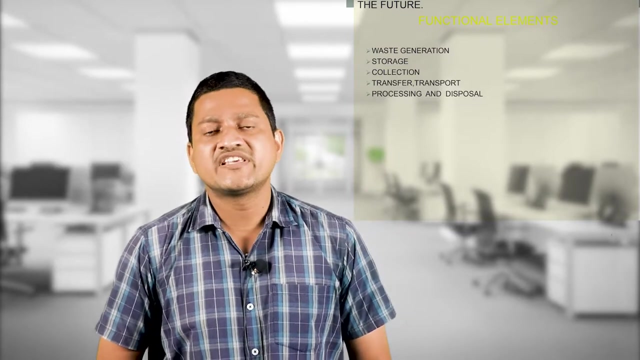 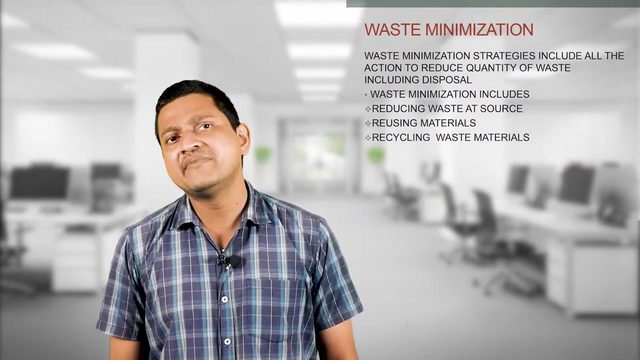 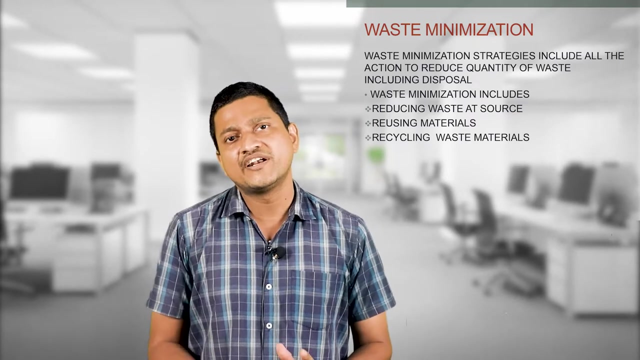 main functional- mainly five functional elements are there in the soil waste management objective. that is, a waste generation, storage of the store, waste collection, transport and transit transfer, processing and disposal. these are the different steps. then waste minimization: waste minimization strategies include all the action to reduce quantity of waste, include including disposal. 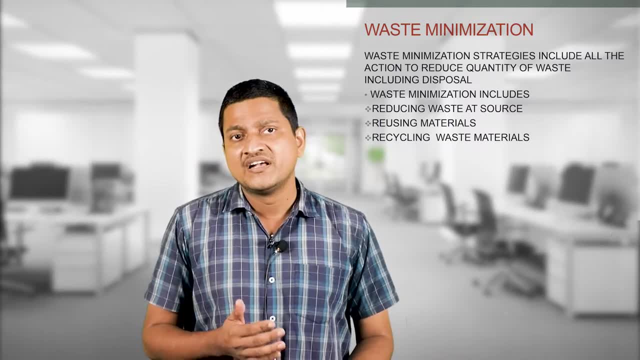 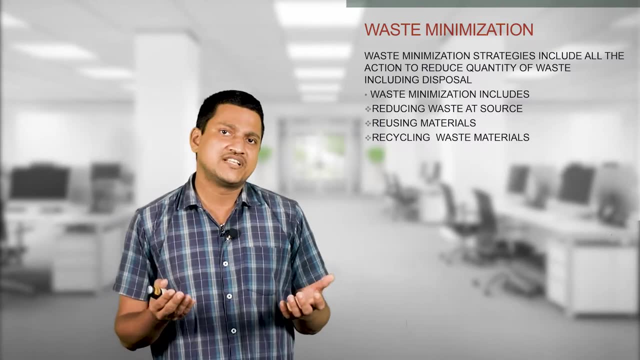 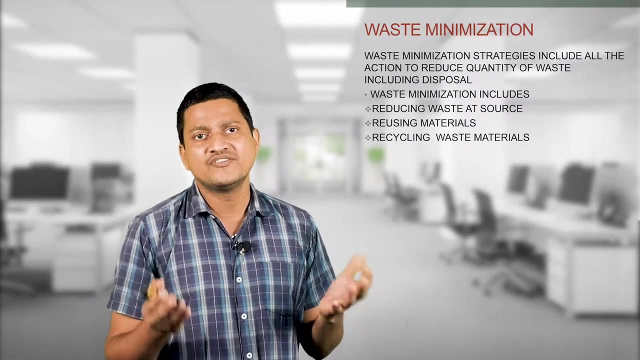 waste minimization, including reducing waste artist source. that means we can reduce the amount of waste at the source. that is, a where it can be original, that is a source of salt waste, for example, in the cardboard box. we can. it can be reused again and again. the packaging paper will be. 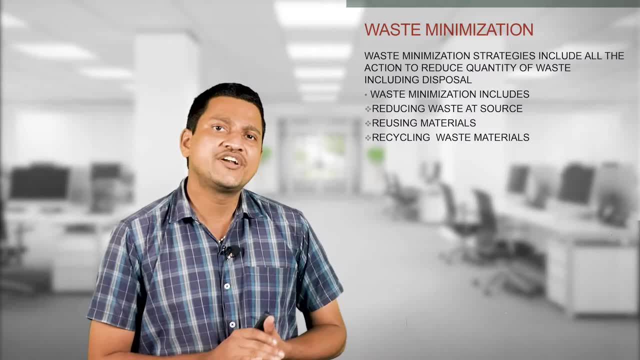 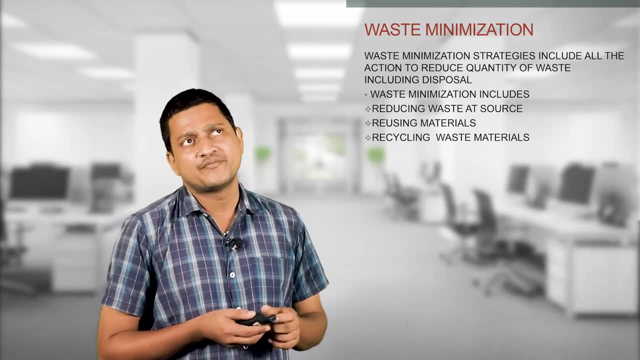 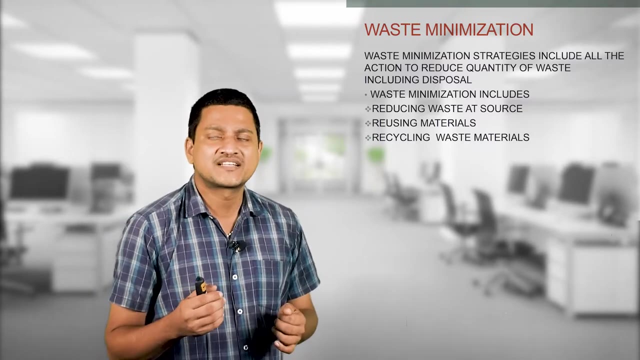 one of the minimize or reduce, then a reusing material. another aspect of waste minimization: they are, you see, once, for example, we can use a shot in our home, it can be used for other type of washing, etc. etc. you some. then recycling of waste material. again, the plastic bottles can. 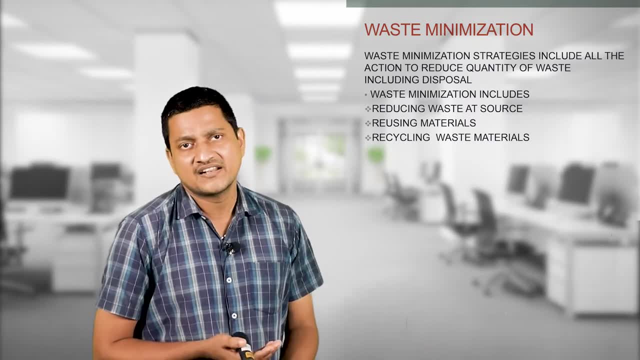 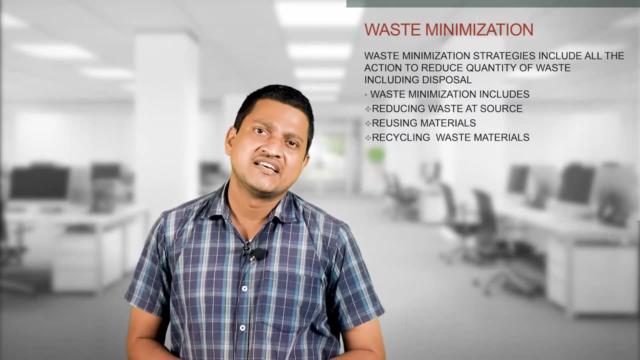 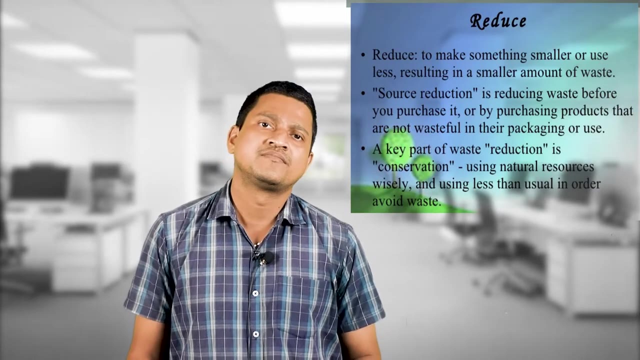 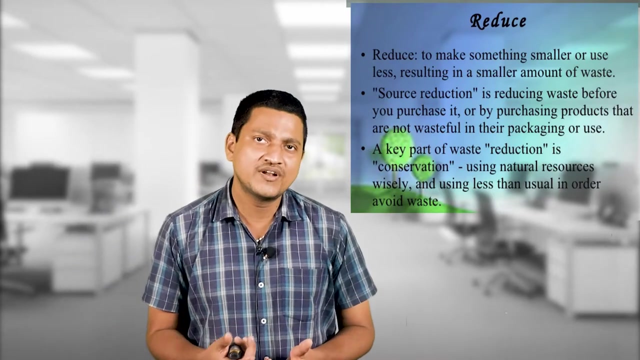 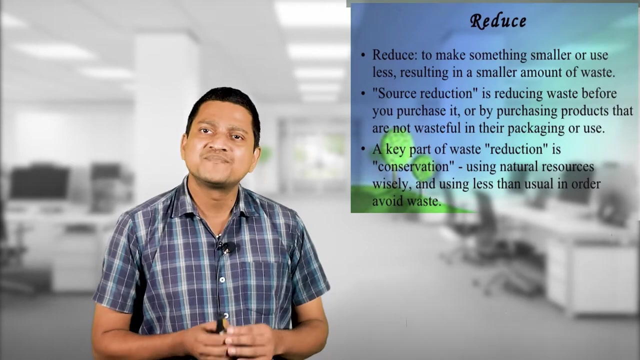 be recycled back to again other products. that is a recycling. there are waste minimization, including reducing based at source, reusing materials, recycling waste material. then what is reduce? reduce to make something smaller. to make something smaller is the meaning of reduce or useless uh, resulting in a smaller amount of waste. in the case of uh water. we. 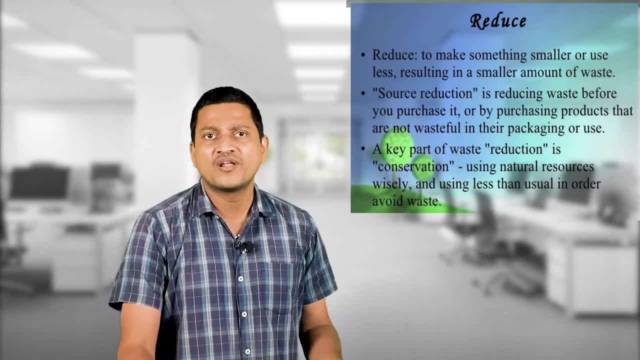 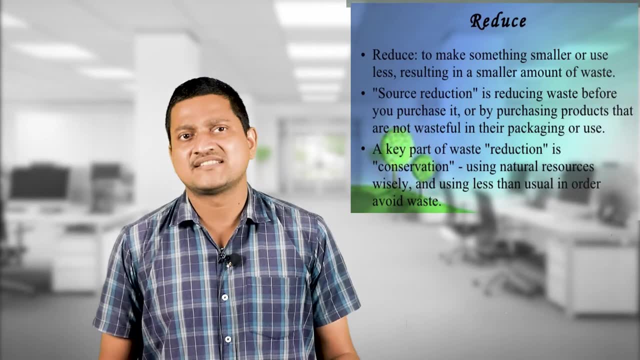 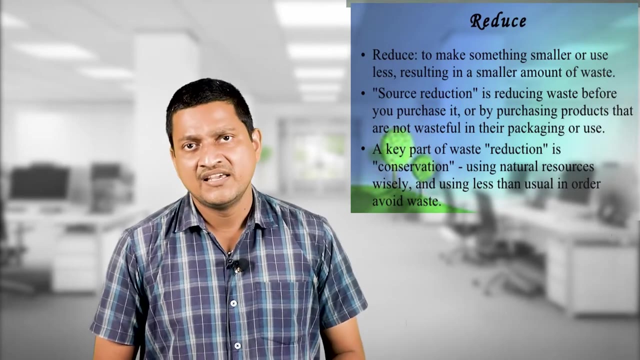 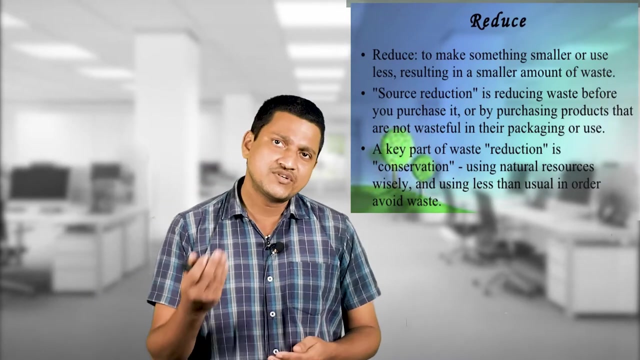 should have, we should produce, can we produce is at a reduction, etcetera. what use? less, smaller, more waste. because you know, reduce means usage can be reduced by a small amount of usage. that is, a reduce means to make something smaller or useless. use less, uh, resulting in a smaller amount of waste. source reduction is reducing width before you purchase it. 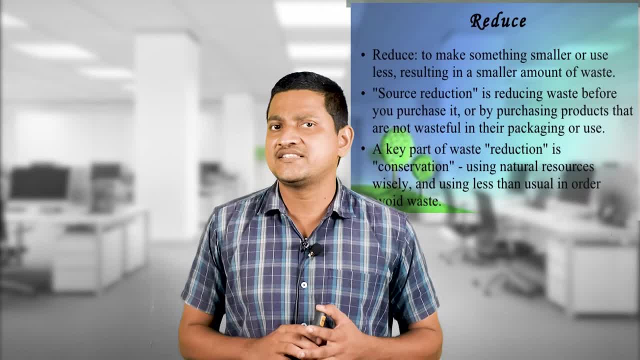 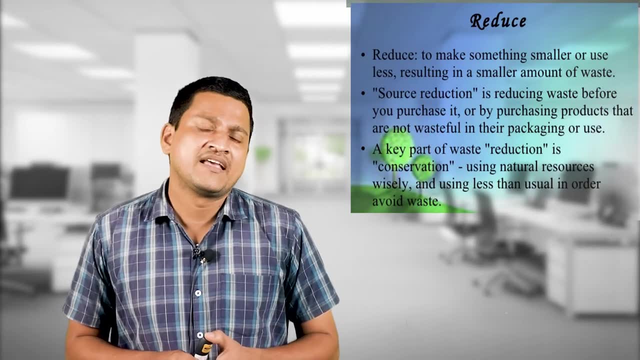 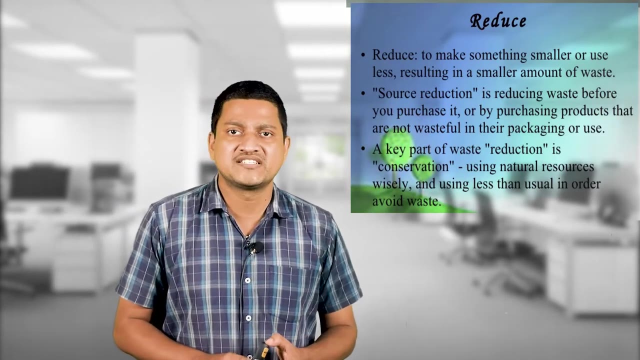 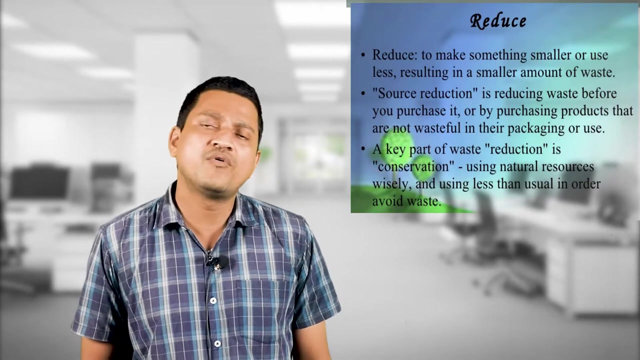 then another component, waste reduction, is a source reduction- purchase it or by purchasing products that are not wasteful in their packaging or use. A key part of waste reduction is conservation. Conservation is important to reduce the waste, Using natural resources wisely and using less than usual in order to avoid waste. 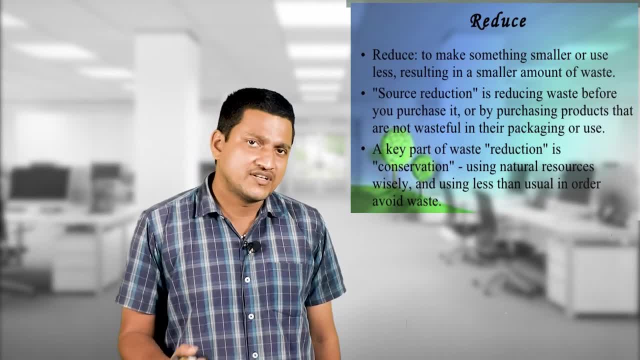 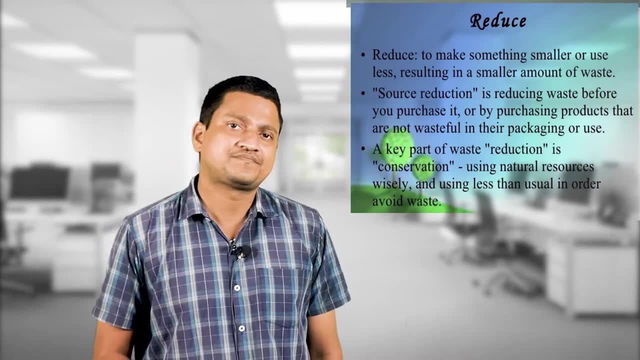 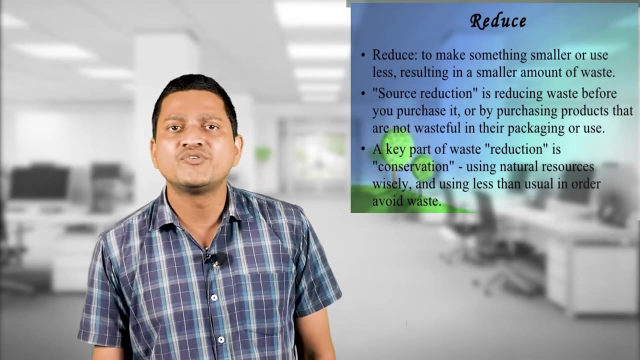 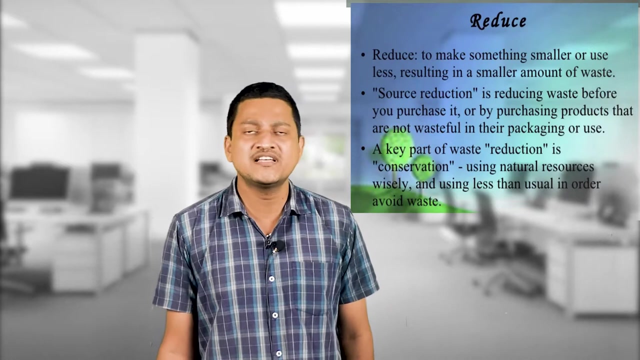 That means we can. sustainable utilization of resource is very important to reduce the amount of waste that can be reduced. Next aspect of second R, that is, first R: the reduce. Reduce means to make something smaller or use less. That is in this reduce, the important point is source reduction. 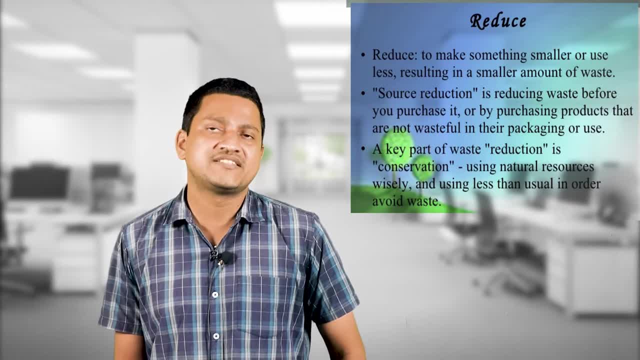 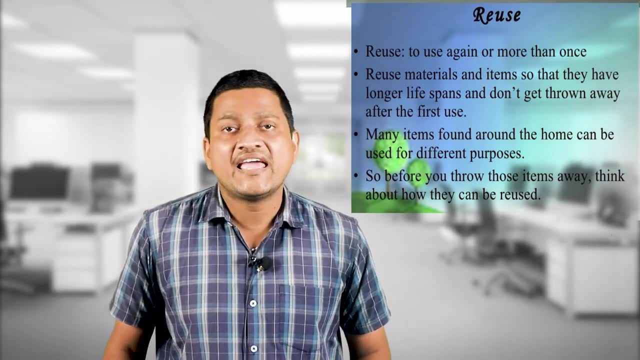 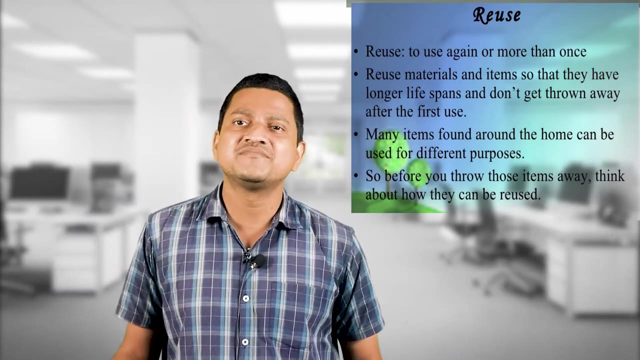 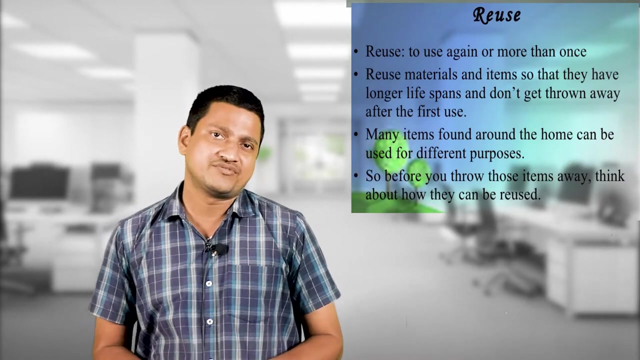 Source reduction means is reducing waste before you purchase it. Second one is a reuse. Reuse means to use again or more than once. Reuse material and item so that they have longer life spans and don't get thrown away after the first use. 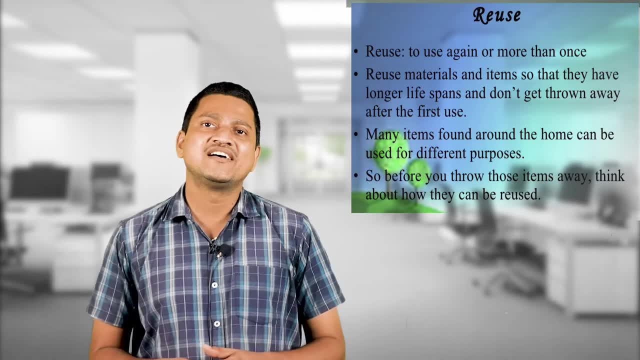 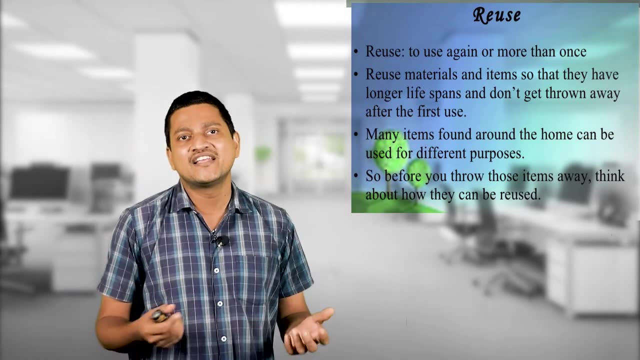 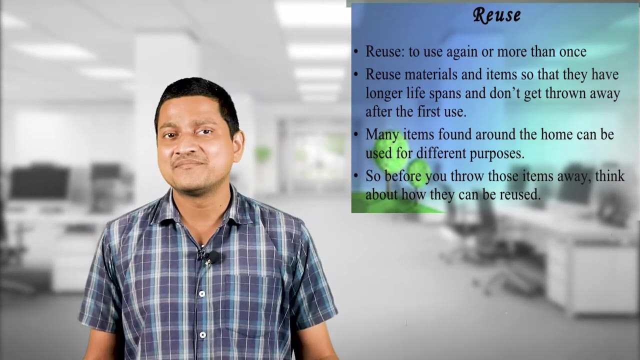 In. nowadays we use mask for protecting against the corona virus. There are some people who use mask. Some people is can be reuse again and again and again for the minimization of waste Many item. is it correct or wrong to use more time in a single mask you discuss? 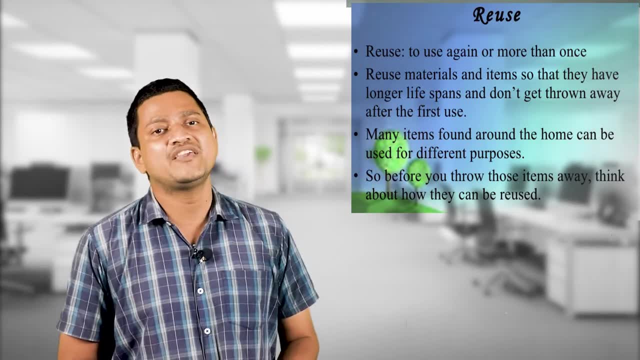 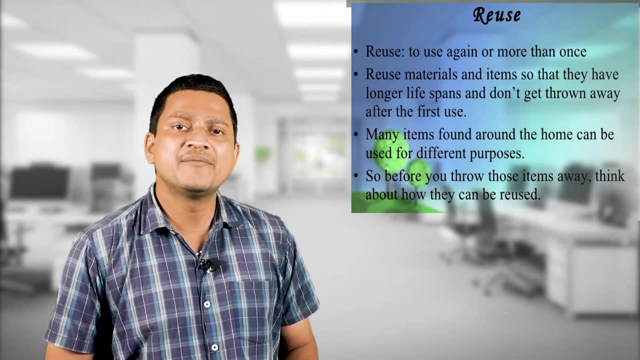 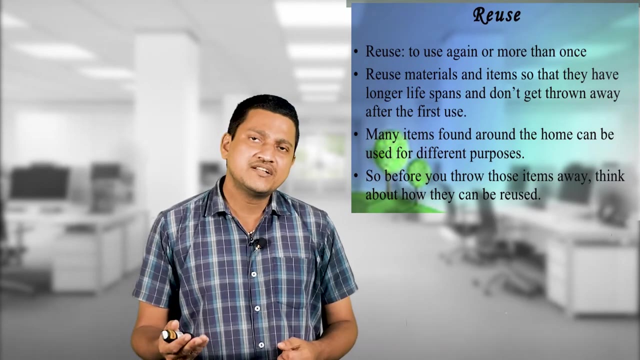 Many items found around the home can be used for different purposes. So before you throw those item away, think about how they can be reused. For example, bottles are used for after there's use bottles, It can be used for decorating household articles, etc. 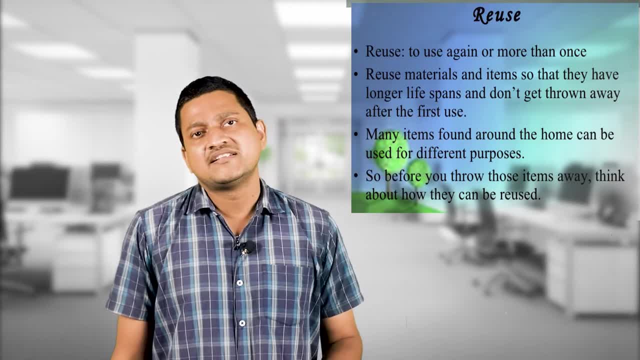 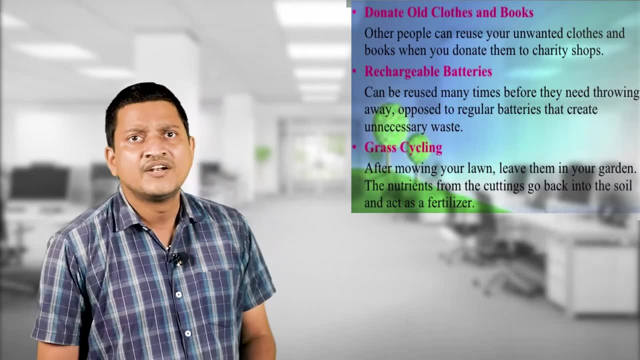 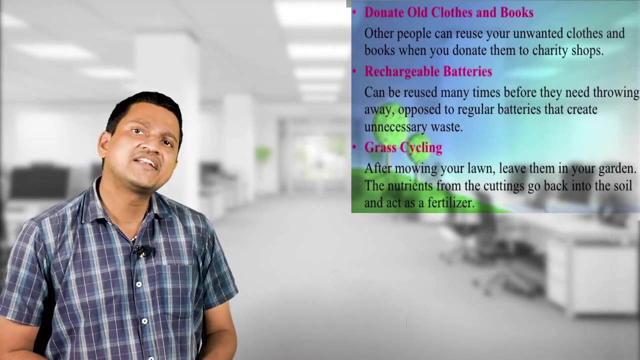 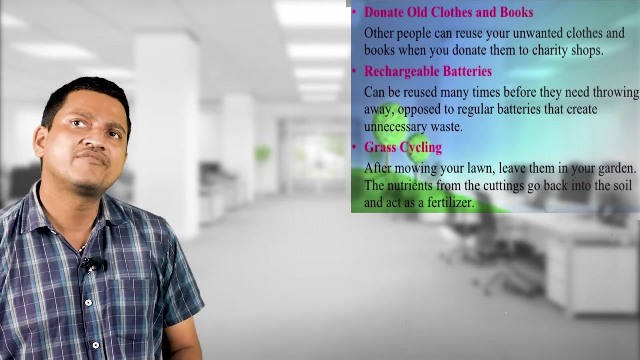 That's the importance of reuse. For example, that's a donate all the clothes and book. It will be helpful for reuse. Other people can reuse your unwanted clothes And book when you donate them to charity shops. That's another method of waste management. 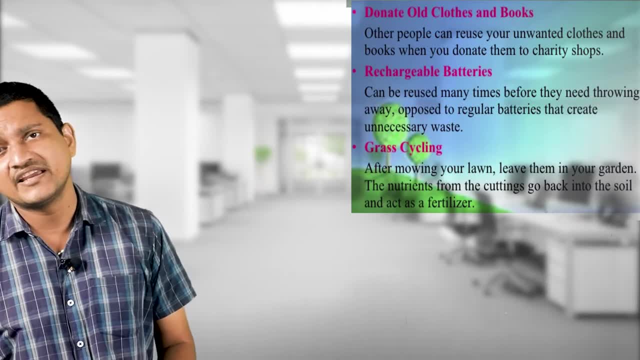 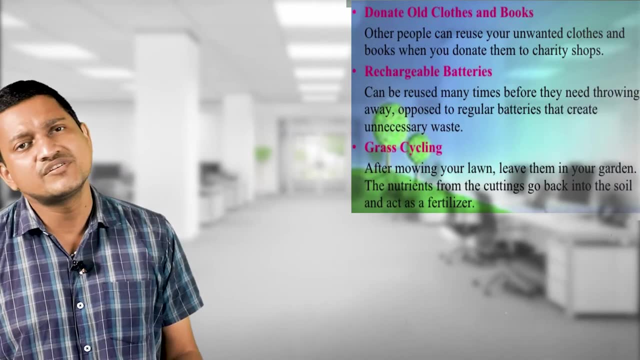 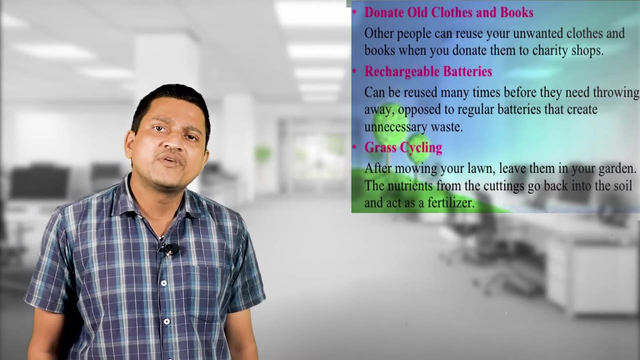 Rechargeable batteries can be reused many times before they need throwing away, Opposite to regular battery that create unnecessary waste. Usage of this rechargeable battery is a reusable method. Then grass cycling: After moving your lawn, leave them in your garden. 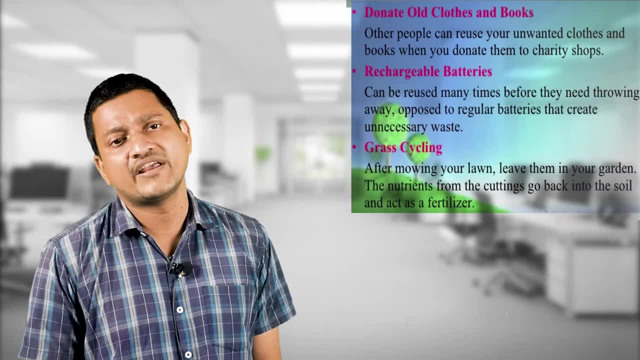 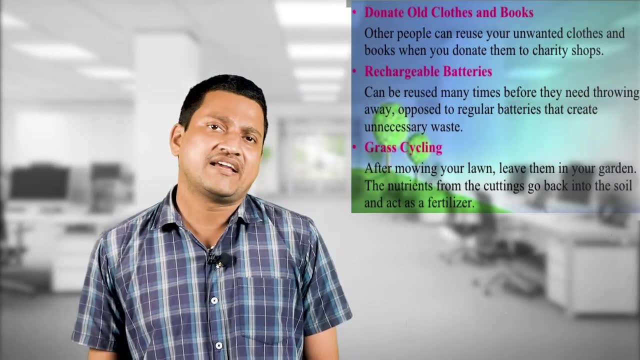 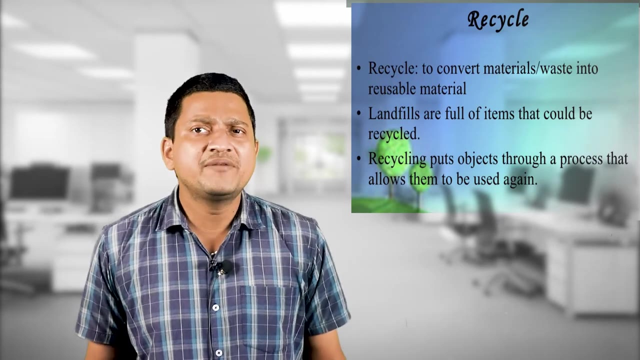 The nutrient from cutting go back to the soil and act as a fertilizer. In Malayalam it is known as Pudavikal. That's how grass cycling is there. Then recycle. Recycle means to convert material or waste into reusable material.